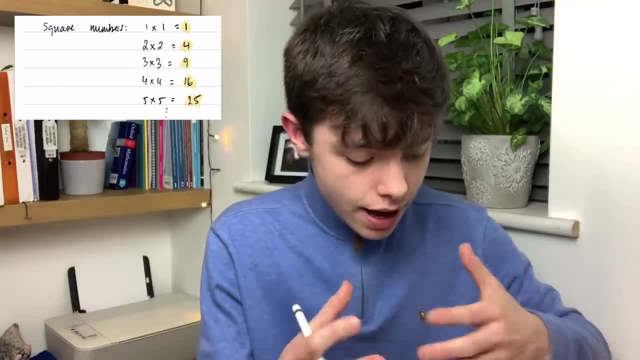 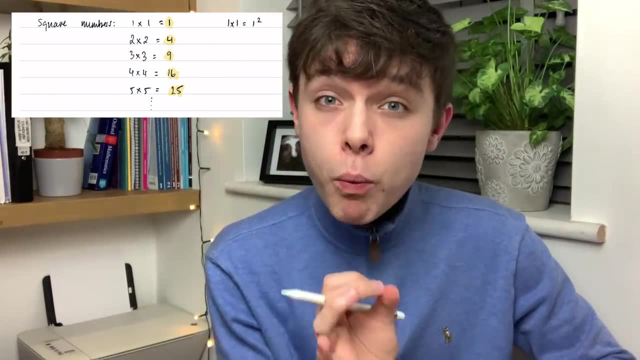 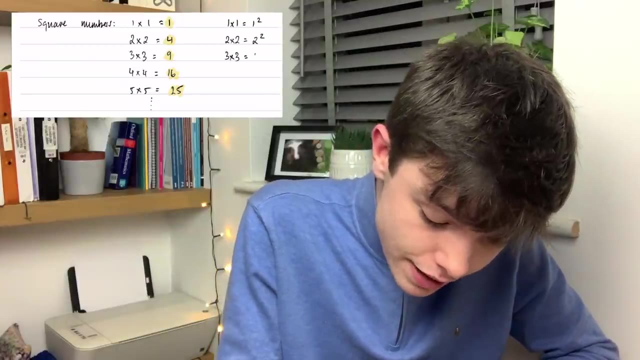 Now here, what we've done is we've done one times one, two times two, three times three, etc. etc. And another way of writing: one times one is one squared On one squared. we just write one with a little two above it, And then two times two is then two squared. three times three is three. 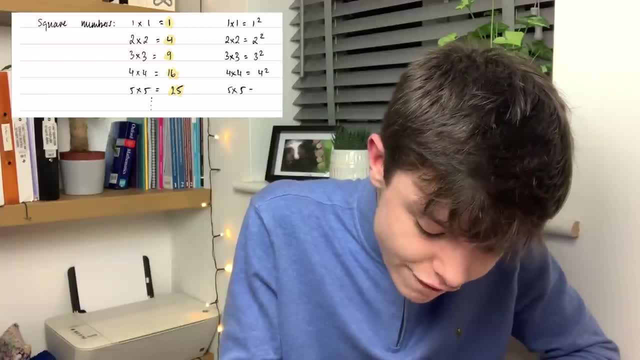 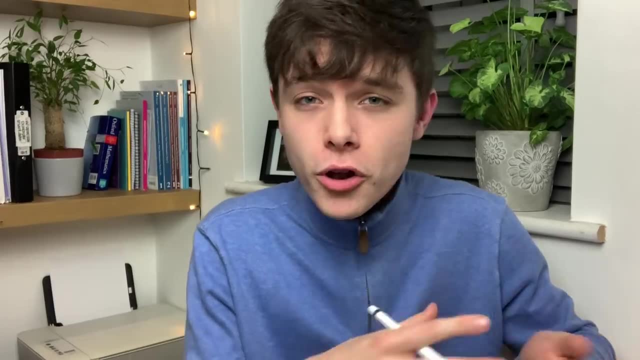 squared four times four is four squared, and five times five is five squared. I'm just letting you know that because as the maths goes on, I might use that abbreviation for doing one times one, two times two, etc. So I'm going to write all the numbers that are highlighted here in a row. 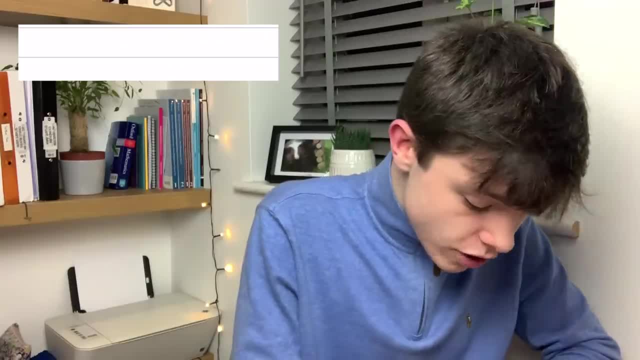 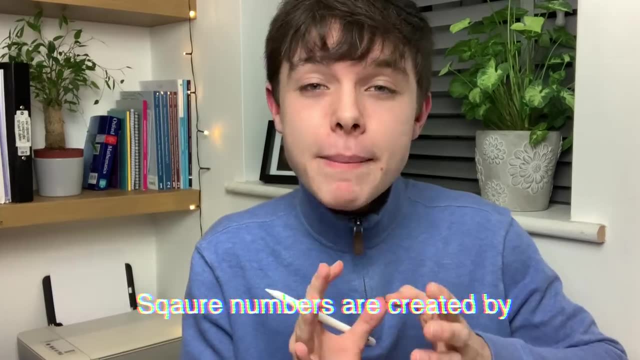 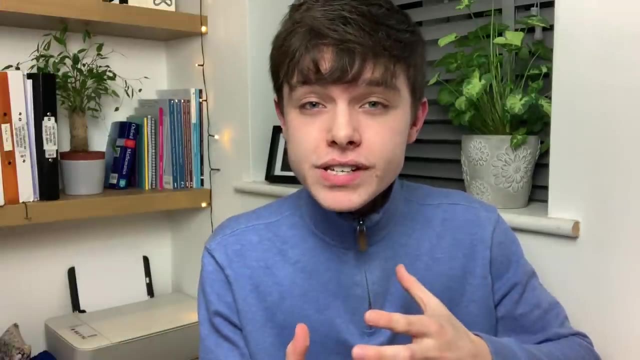 because those are our first five square numbers. So we've got one, four, nine, sixteen and twenty-five. So, to summarise, square numbers are created by multiplying an integer by itself. Now, just like when we add numbers together, we can do the inverse of that, which is to subtract numbers. 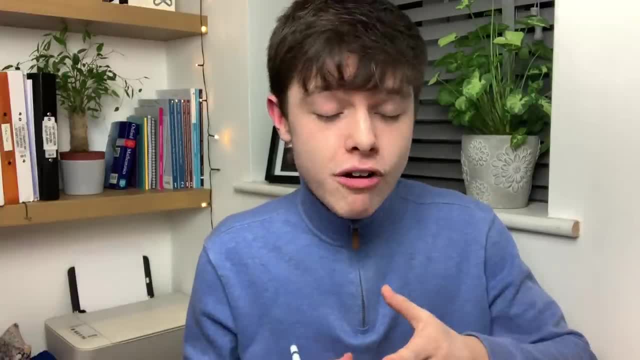 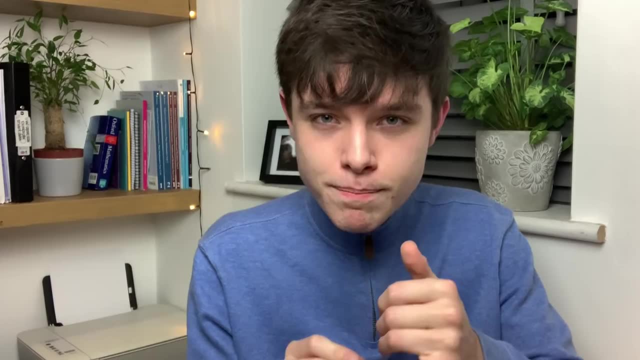 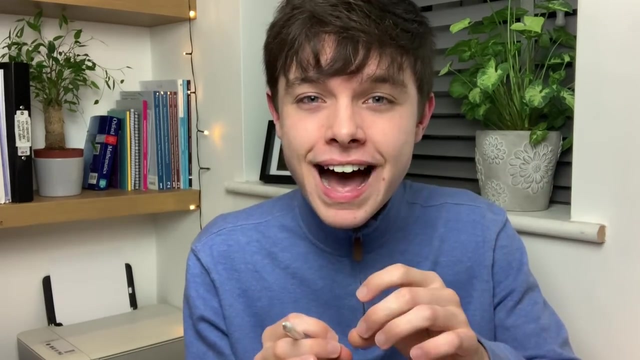 The inverse just means to undo something. So, for example, if we divide, the inverse of dividing is multiplying. So because we've got an inverse for multiplying and dividing and adding and subtracting, somewhere in the world of maths we must have an inverse for squaring and it's called 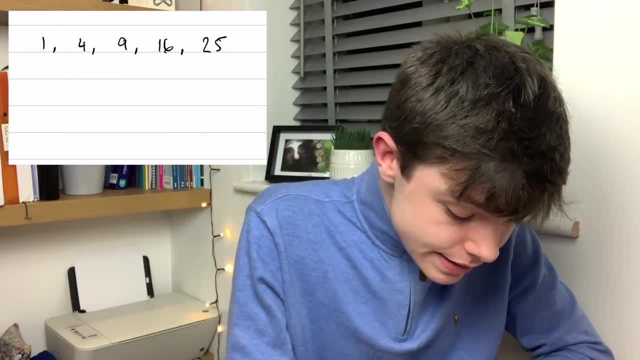 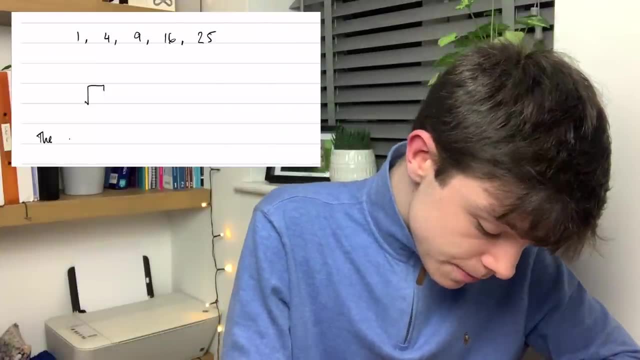 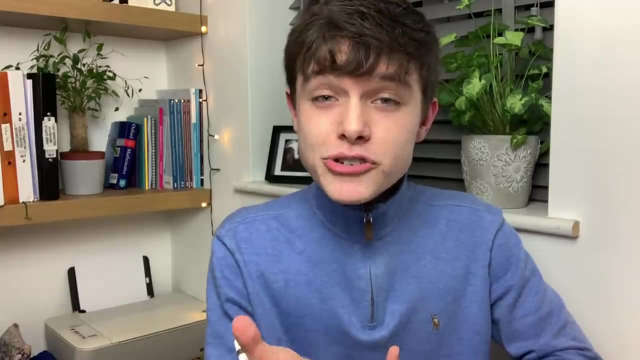 square rooting. The notation for square rooting is that. I don't really know how to explain that. we can just see that that's what it looks like. The inverse, which means to undo or squaring, is square rooting. So let's try that out with a few. 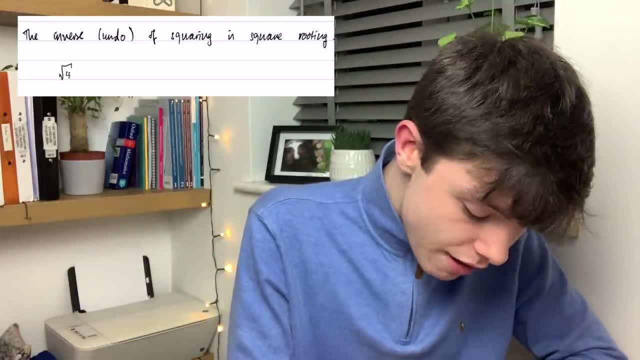 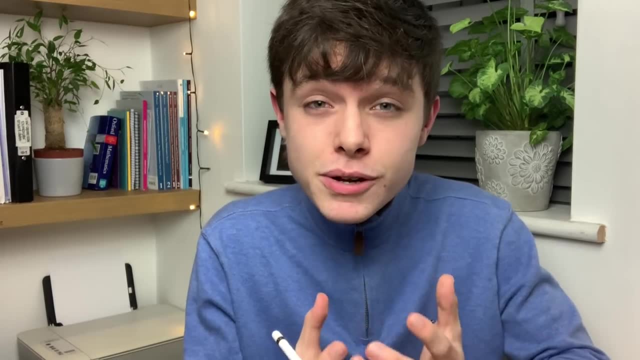 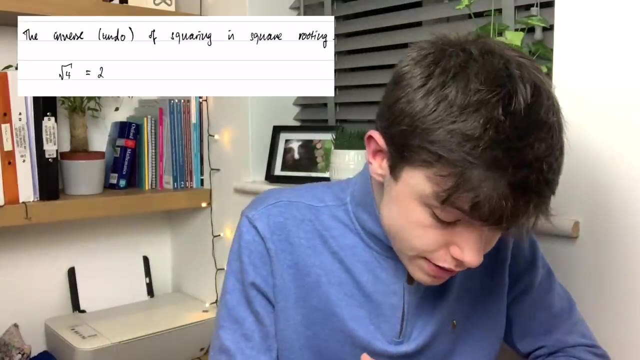 numbers. For example, if we want to work out the square root of four, what we need to think is: what number is multiplied by itself. So what number do we square to give four? And we know that that's two. So the square root of four must be two. If we were to do the square root of, let's say, 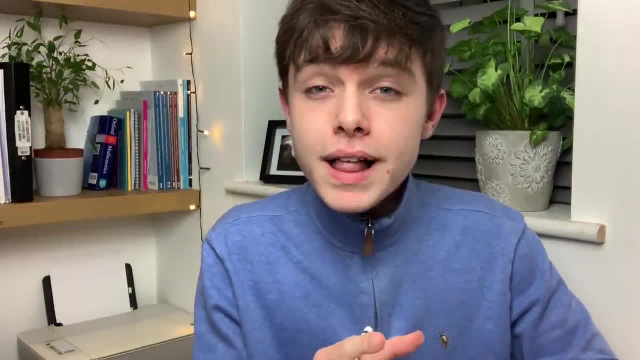 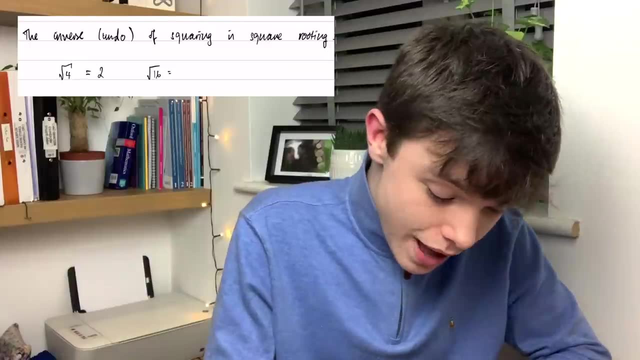 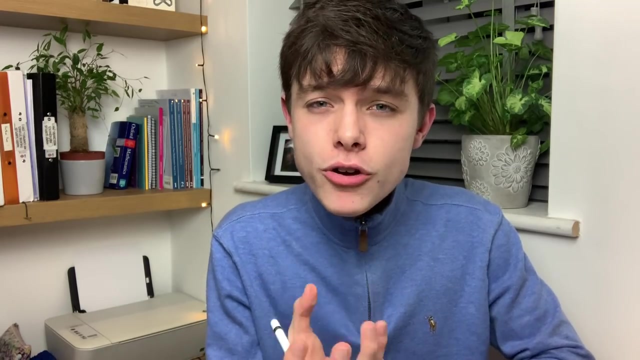 sixteen. we're trying to find the number that multiplies by itself, to give sixteen, And we know that that's four, because four times four is sixteen. So the square root of sixteen is four. Let's have a go at the square root of one hundred. Again, we need to think what number is squared. 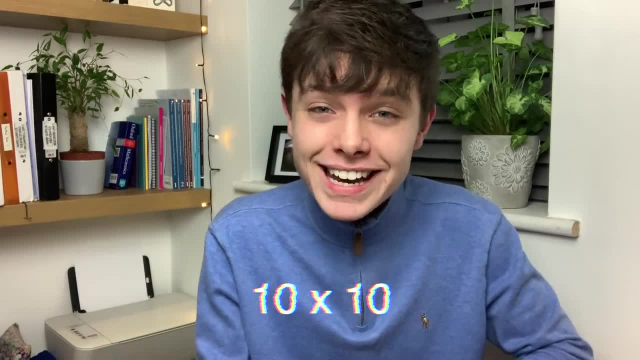 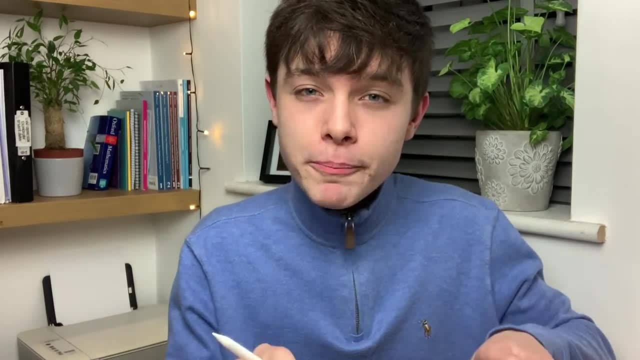 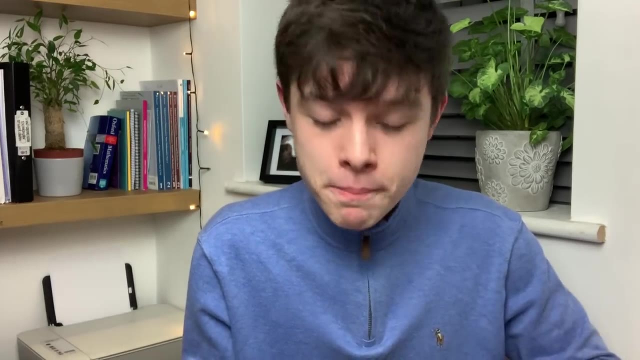 to give one hundred, Well, that's ten, because ten times ten is a hundred. So the square root of a hundred is ten. Now, what we've just done, there is square rooted square numbers. But what happens if we square root, let's say, thirteen? Because thirteen isn't a square number? 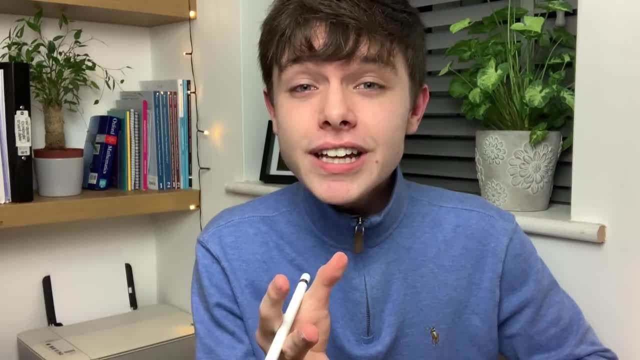 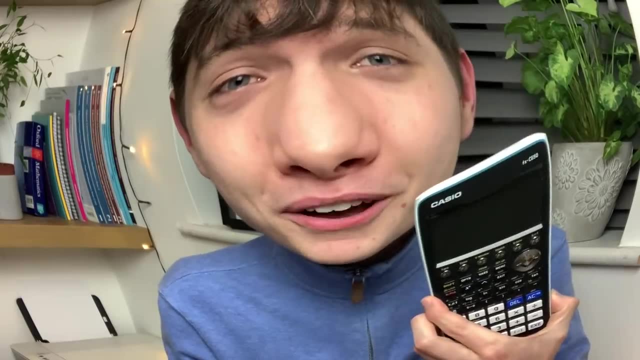 Well, let's try it: Square root of thirteen. If you've got a calculator or you know where a calculator is, go and get your calculator. If you've not got a calculator, I'll do the work for you. So what we're going to do is we're going to do the square root of thirteen on the calculator. 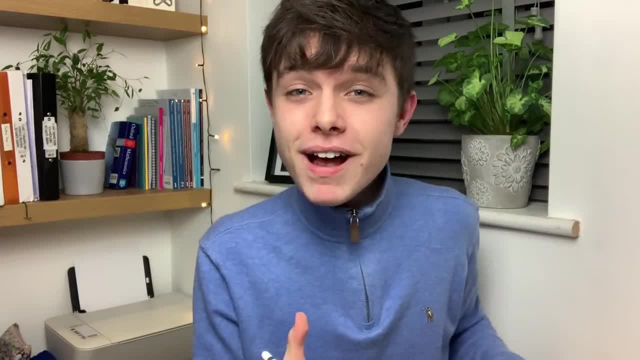 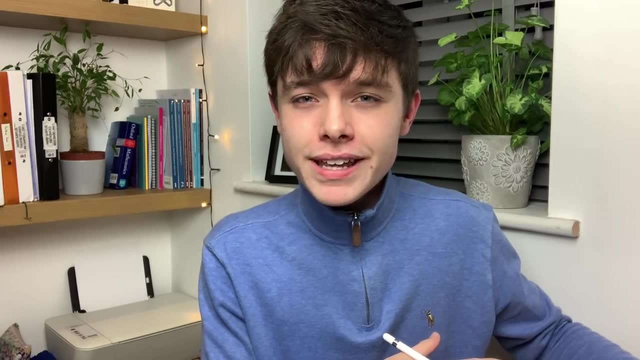 So square root and then thirteen, And when you press equals on your calculator it just gives you the square root of thirteen. So it's not really that useful when you put it in your calculator. Now the reason your calculator does that is because the square root of thirteen is an irrational 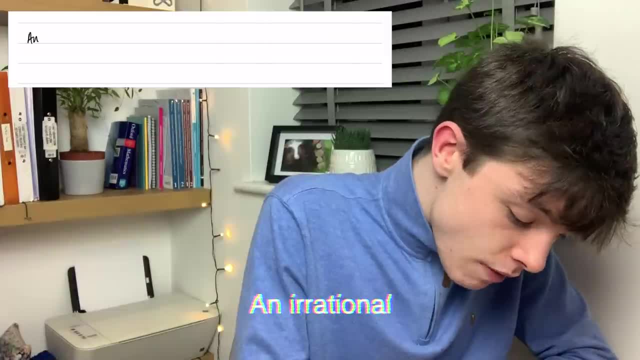 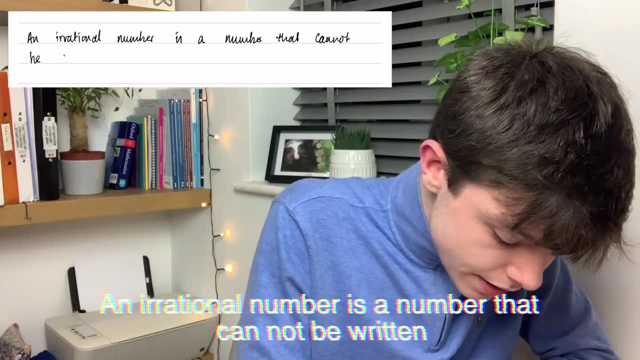 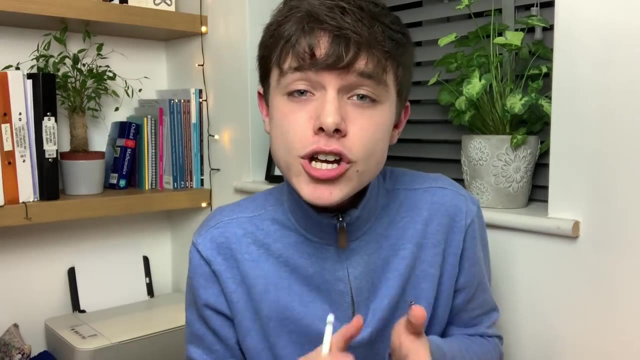 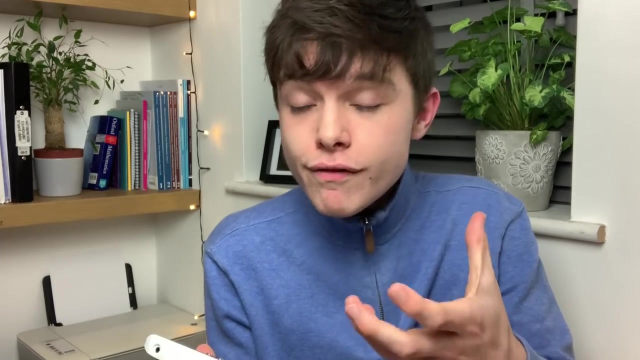 number. Stop. We need a definition. An irrational number is a number that cannot be written as a fraction. So root thirteen cannot be simplified any further. It can't be written as a fraction, So therefore it's irrational If we were to press s to d on our calculator, which means to convert that number into a decimal. 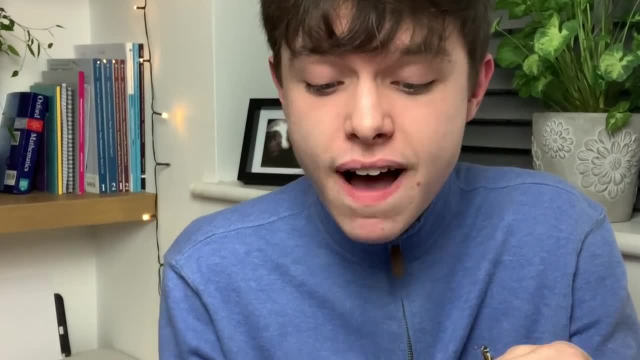 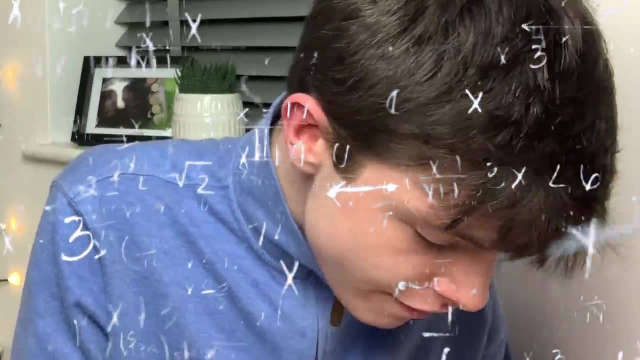 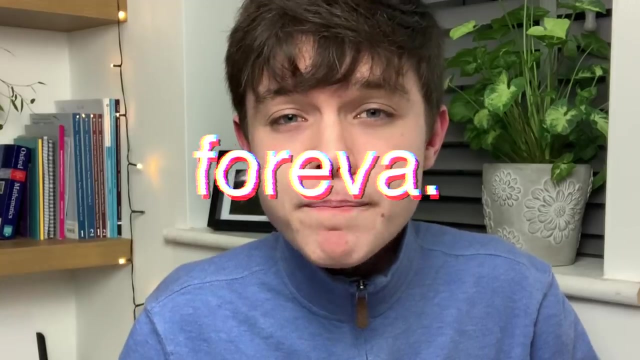 we can see that the calculator gives us 3.6055 and that carries on. So root thirteen is 3.605551 and that carries on, And in fact those decimal places will carry on forever. Now, from looking at the two ways we can write root thirteen, I think that you'll agree with me. 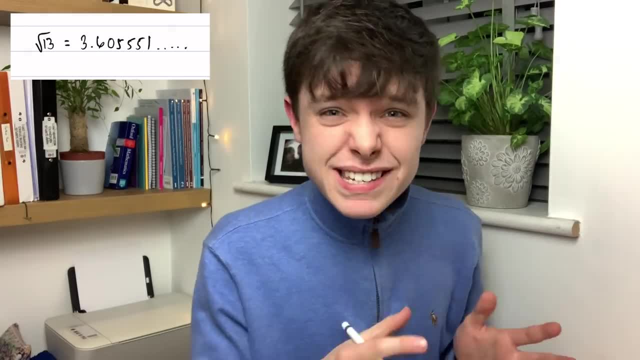 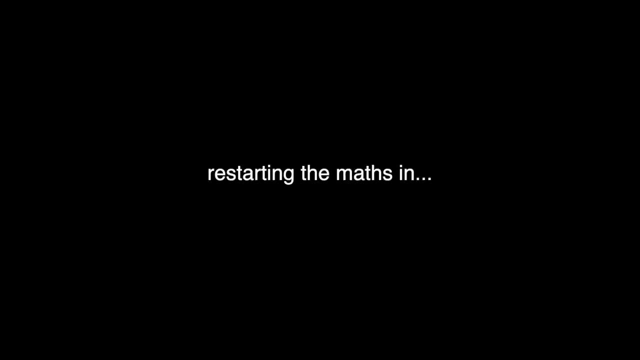 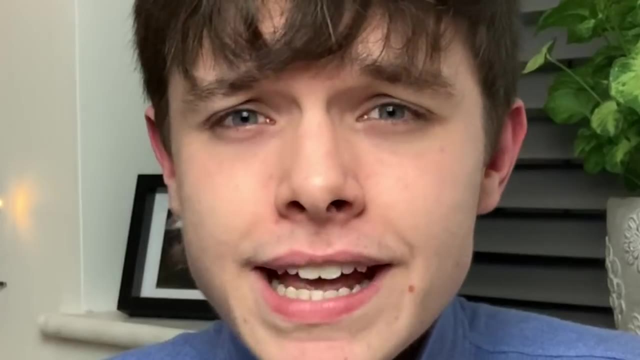 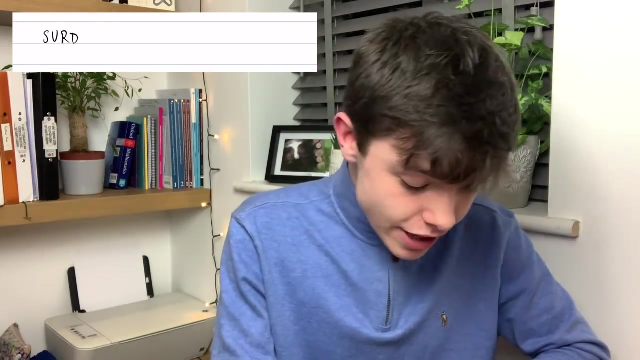 Writing it root thirteen is much better than writing it as the decimal equivalent. Now I'm going to introduce a new word. If you've never heard of this word before, then it's new. I'm going to introduce the word surd, Spelt s u r d, And the definition of a surd is a number. 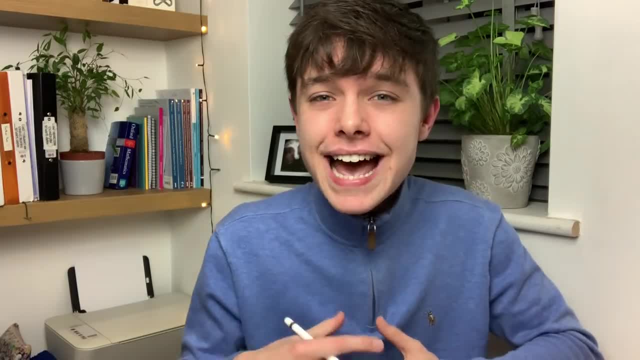 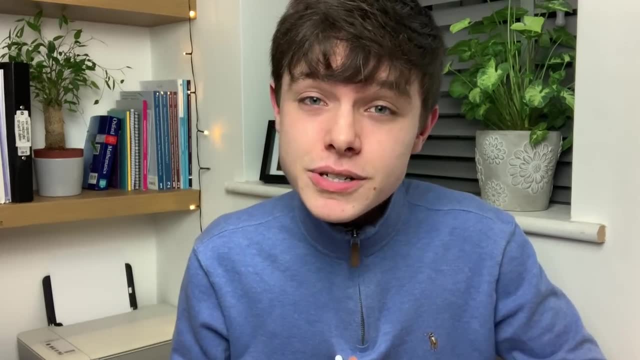 in root form And it can't be simplified Now. root thirteen is just root thirteen. We can't simplify that any further. So root thirteen is a surd. So to summarise, a square number is found by multiplying a number by itself. 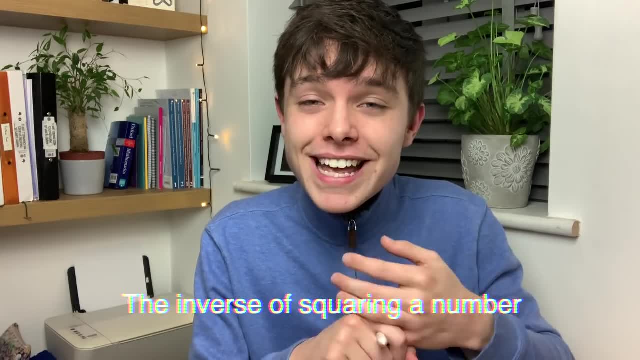 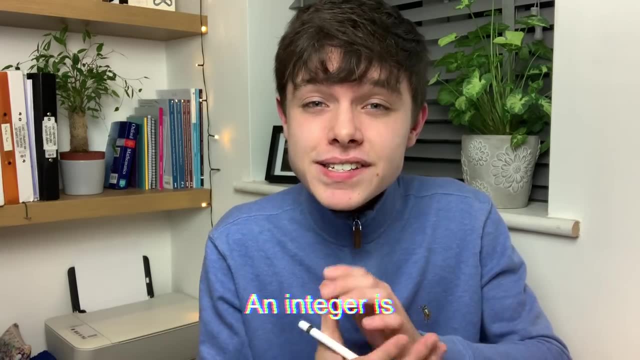 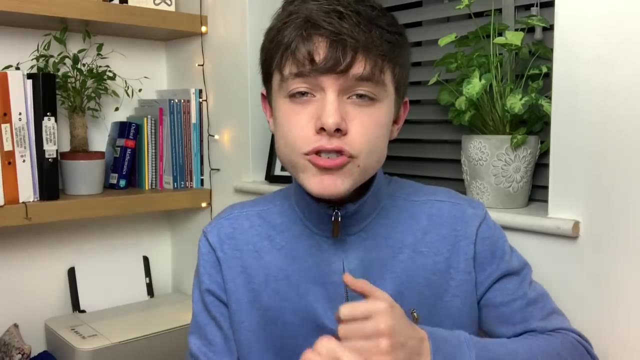 The inverse of squaring a number is square rooting. When square rooting a square number, your answer will be an integer, And an integer is a whole number, And when you square root a non-square number, your answer will be a decimal. So we have tried square rooting square numbers And we've tried square rooting non-square numbers. 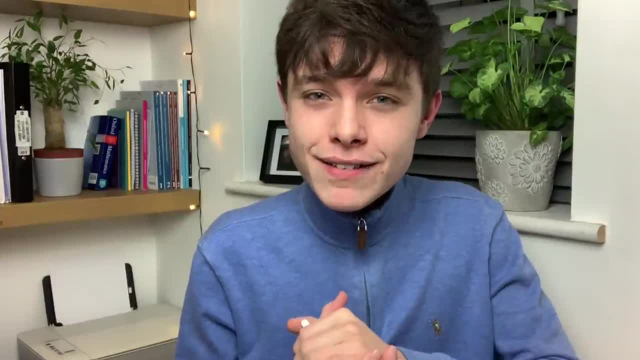 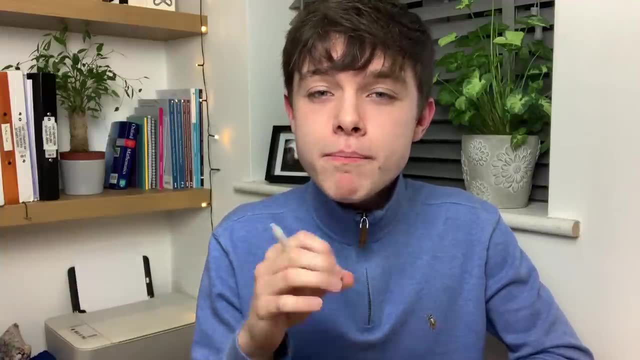 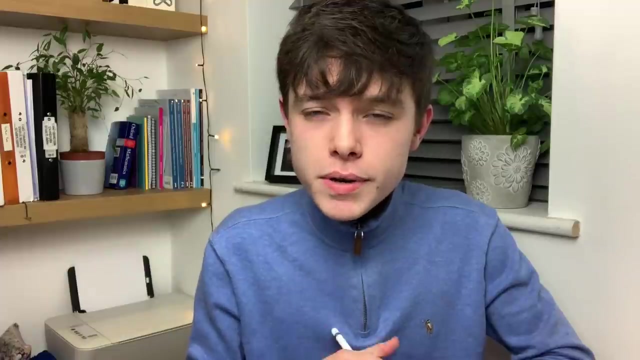 What about if we square root negative numbers? Let's take, for example, negative one. Now remember, when we're square rooting, we're trying to find the number that multiplies by itself to give the number under the square root. So what I'm trying to find here is what two numbers multiply together to give minus one. 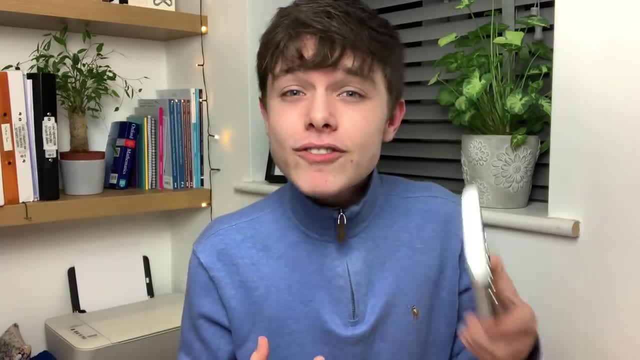 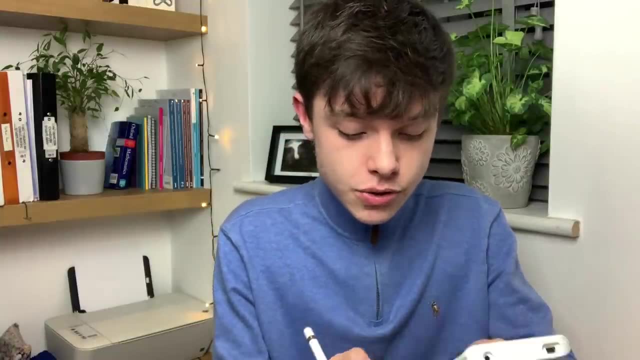 Well, I don't really need to do that thinking here, Because I've got this device. It's a calculator. So what I'm going to do is in my calculator I'm going to put in the square root of minus one. Now, when I do that, my calculator says non-real error. 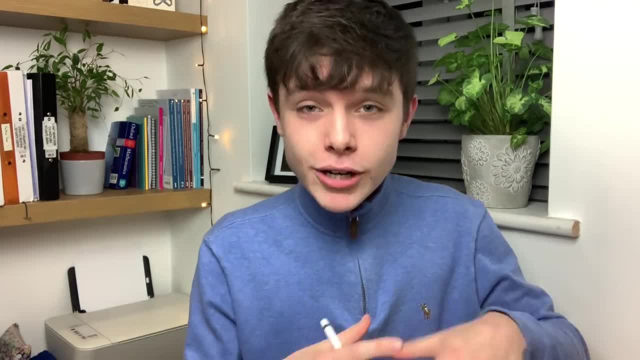 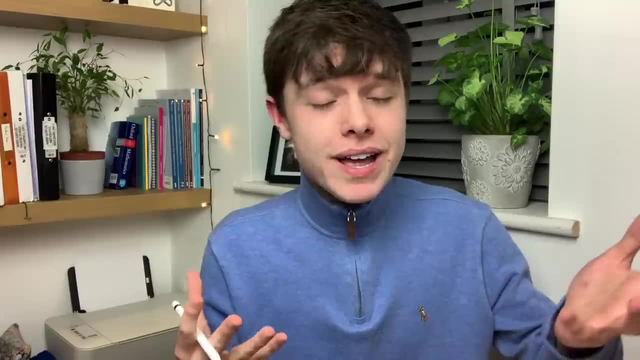 Your calculator might say math error, But it doesn't matter what it says, because we've got an error. So does that mean maths is broken? Does that mean we all leave maths And we can't find anything else about maths? No, Because my calculator says non-real error. 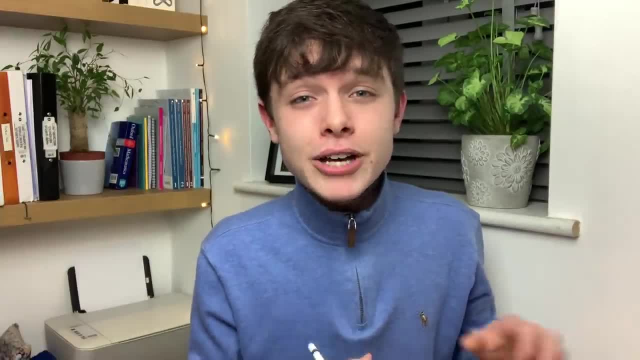 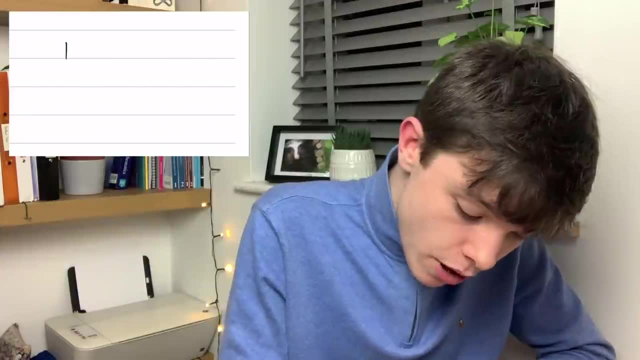 I'm going to try and do it myself, because my calculator might not be able to do it. So let's try and find a number that multiplies by itself. to give minus one, I'm going to put a box, and another box equals minus one. 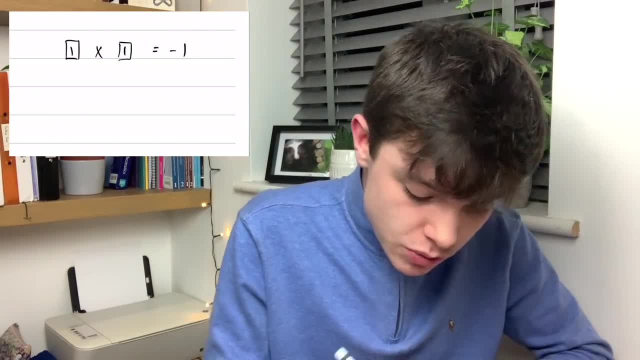 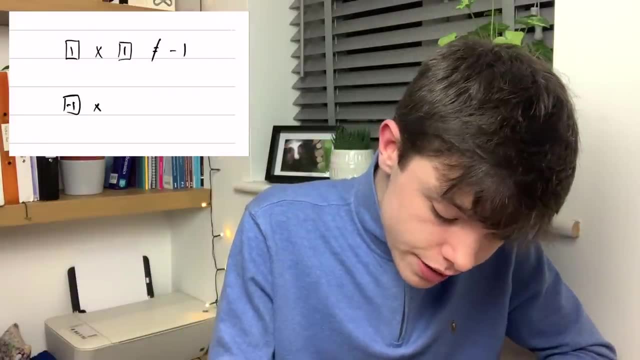 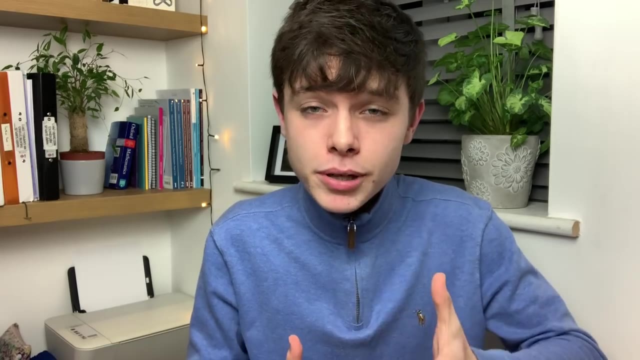 So I'm just going to try one One times one, of course, equals one, So it doesn't equal minus one. Let's try minus one times minus one. Does that equal minus one? Well, no, Because a minus times a minus is a plus. 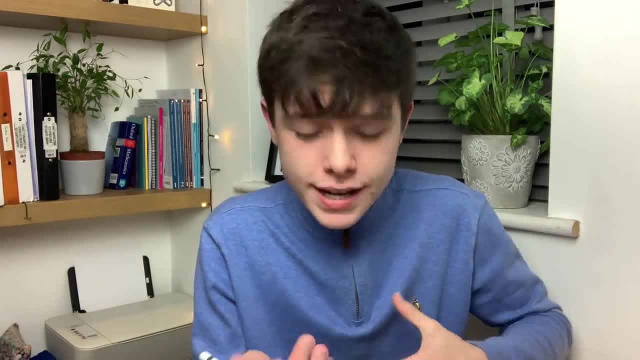 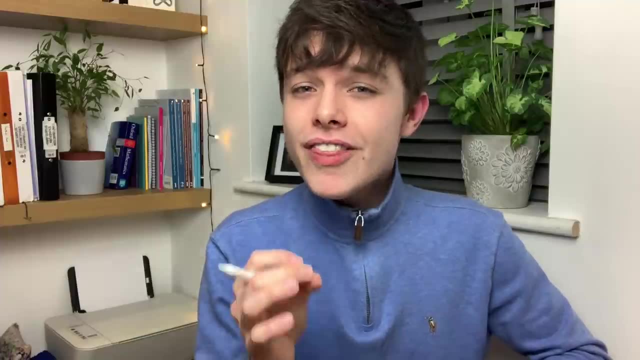 And one times one is one, So minus one times minus one is one, So not minus one. You could try many other numbers as well, but I'm going to save time and tell you that there isn't a number that, when you multiply by itself. 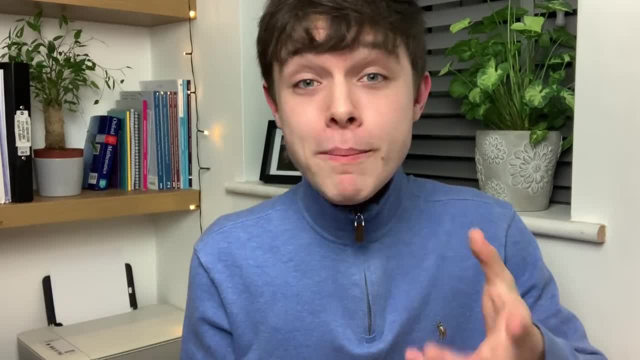 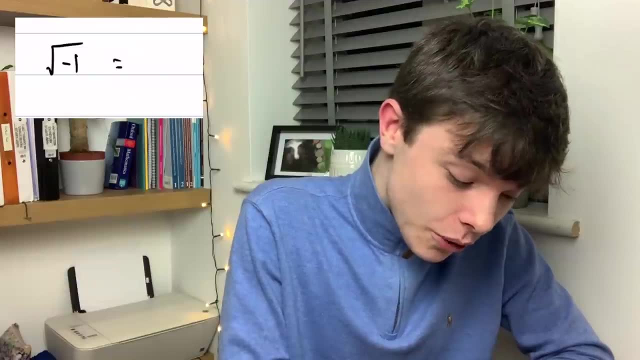 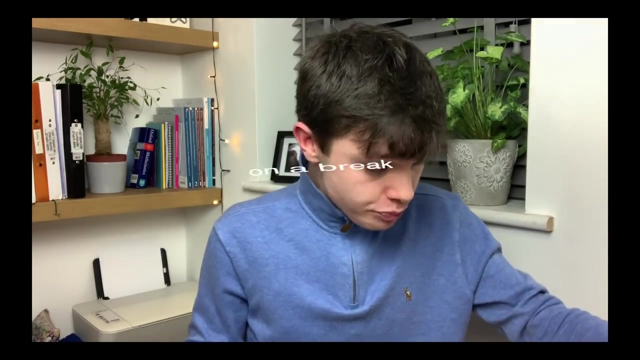 gives minus one. So what do we do? We make up a number, And the number that we make up is i. The square root of minus one is equal to i. Yes, this is getting confusing, so let's take another break. Has everybody refreshed a little bit? 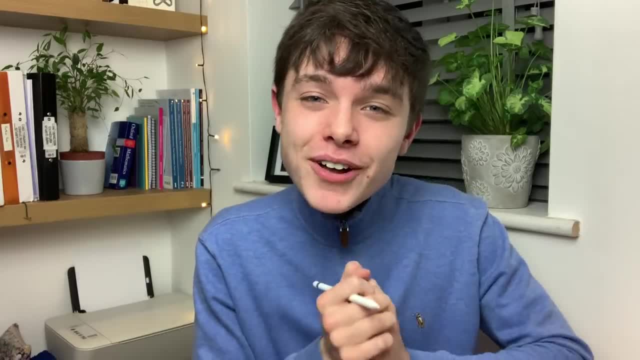 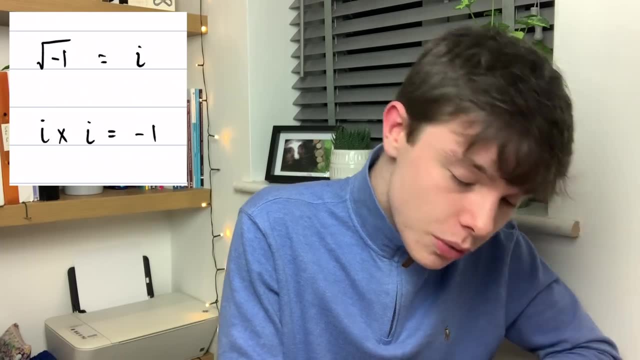 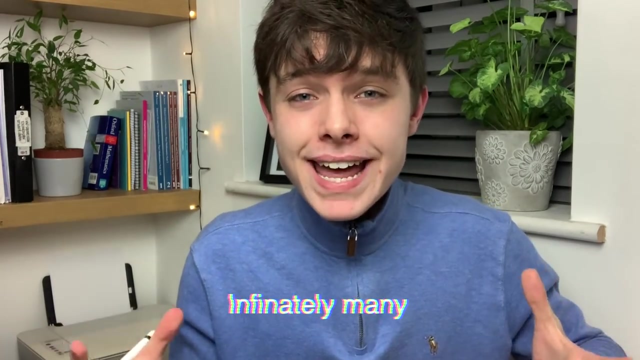 I hope that you have. So in maths we call the square root of minus one i. So what that means is: i times i is equal to minus one, And that is what an imaginary number is. And in fact there are infinitely many imaginary numbers. 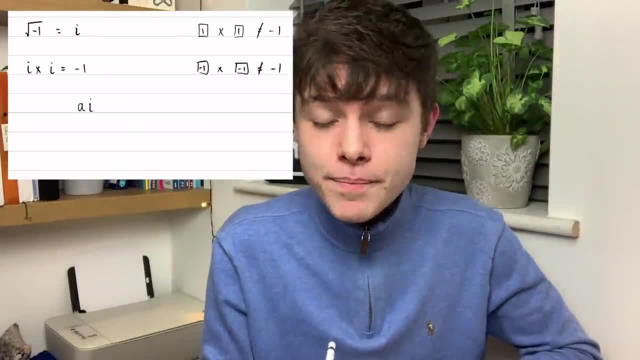 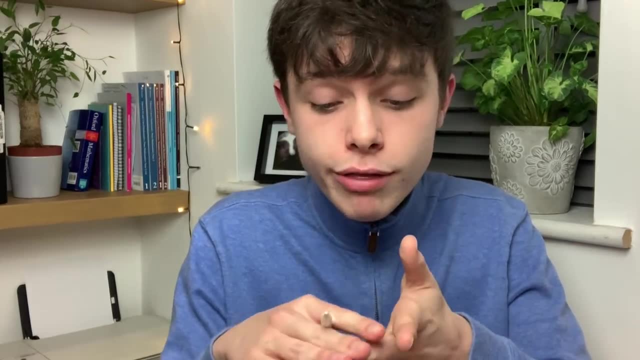 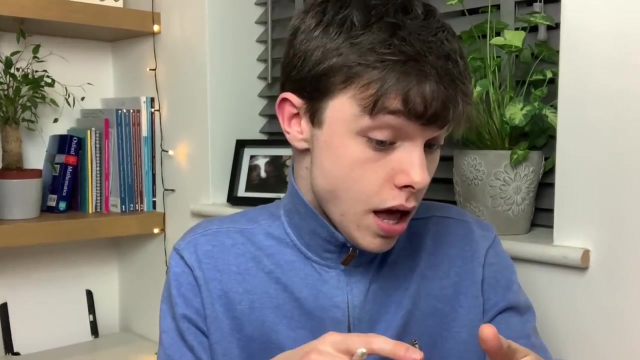 So an imaginary number is in the form ai, Where a is a real number, And what I mean by a real number is one, two, three, four minus sixty-four, minus ninety-two, minus a half, a half, any number like that. 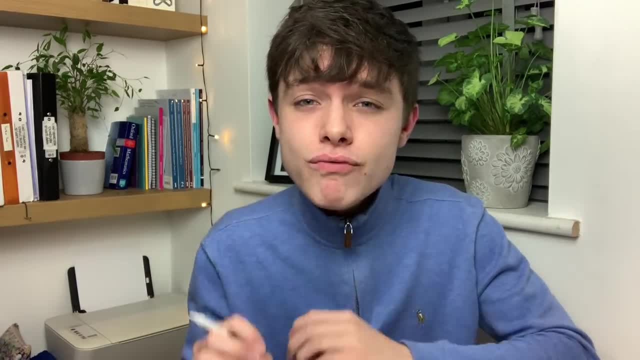 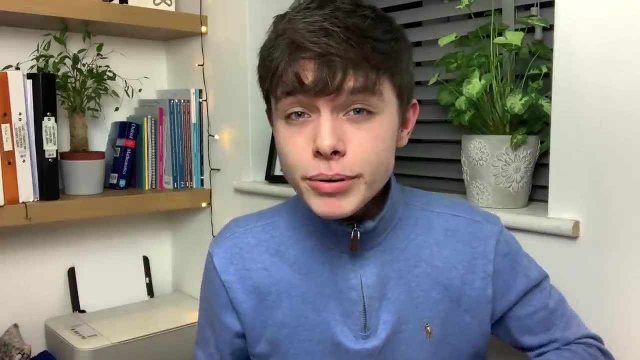 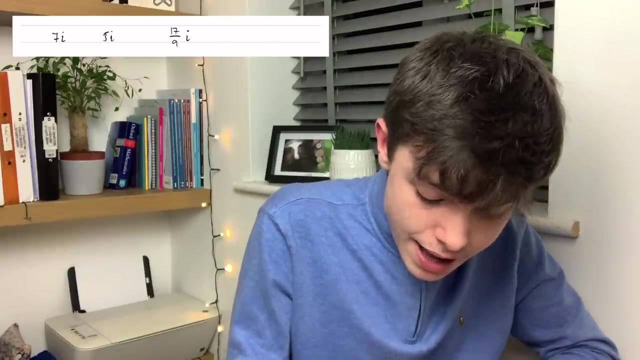 it can be a fraction, it can be positive or negative, is a real number. So some examples of imaginary numbers are seven i, five i, seventeen over nine i minus sixty-three i and seven point five i. Those are some examples. 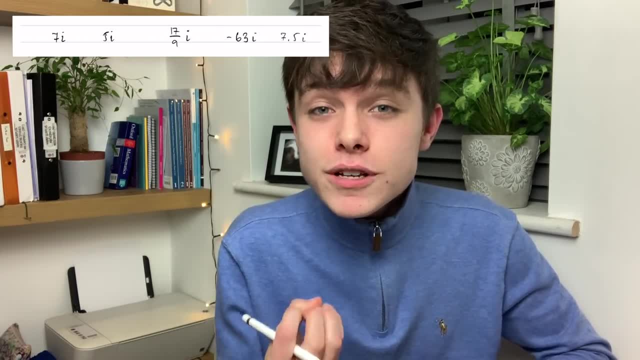 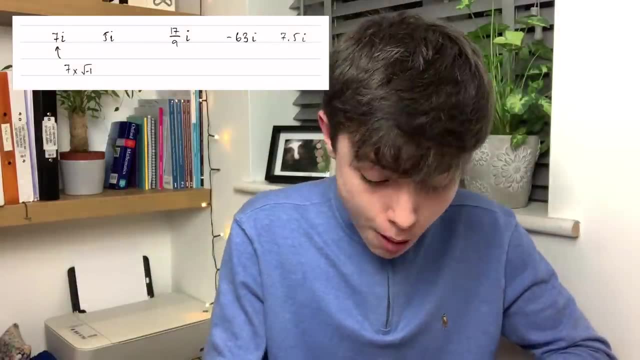 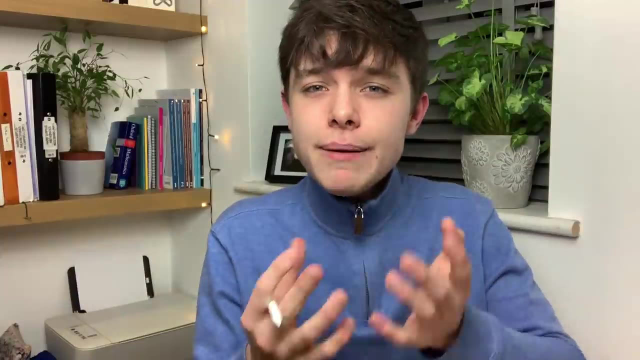 Now remember that the i means the square root of minus one. So what seven i actually means is seven times the square root of minus one, And what minus sixty-three i actually means is minus sixty-three times the square root of minus one. Now I'm sure you're thinking. 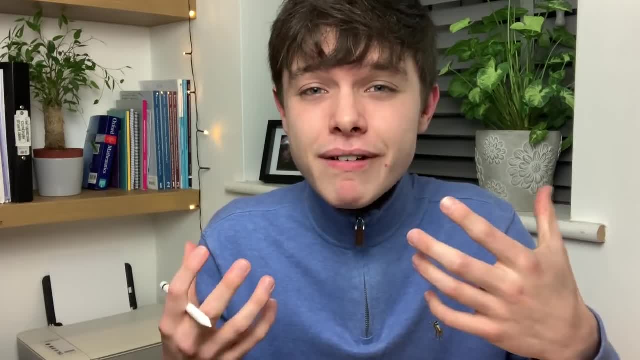 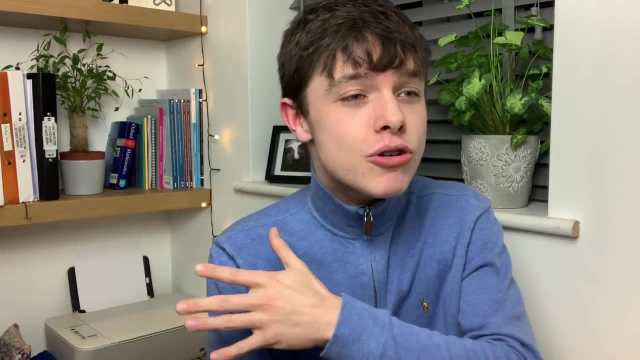 what is the point in all this? Because the title says imaginary, They're not real. There isn't a real value for the square root of minus one. But imaginary numbers come into maths in a whole bunch of topics They come in quadratics. They come under advanced calculus And, surprisingly, they're used in many real life situations, One example being in electricity. That's not where it stops. Imaginary numbers can be added to real numbers to make complex numbers. Now, yes, they say they're complex. 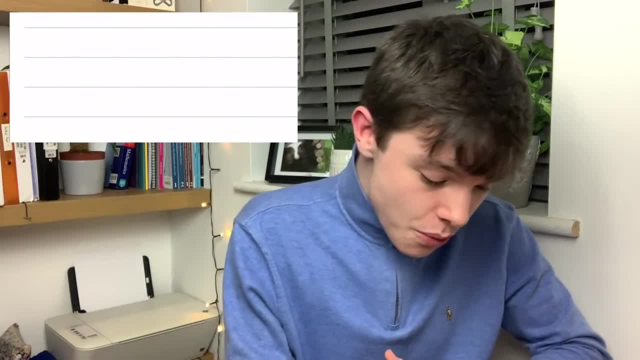 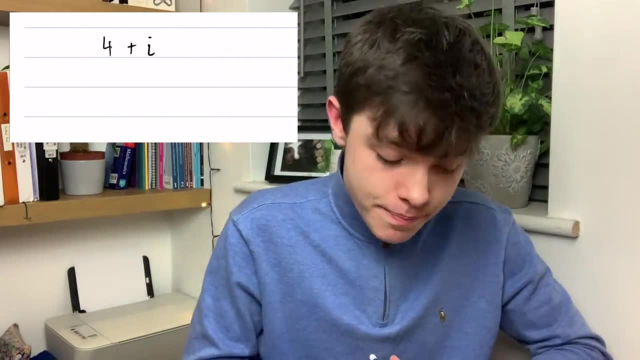 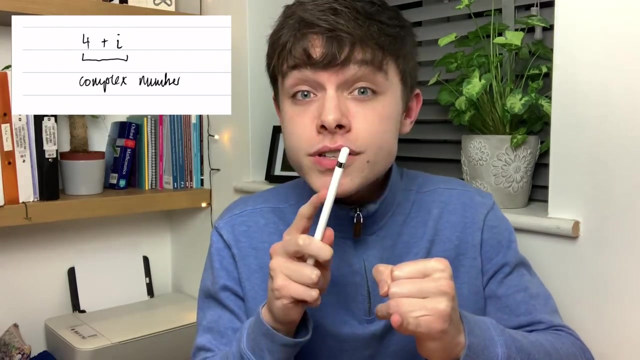 but I'm only going to introduce you to a little bit of them. Let's say we have four and we add to that the square root of minus one, So i That is a complex number. Now, why is it a complex number? Because, like I just said,